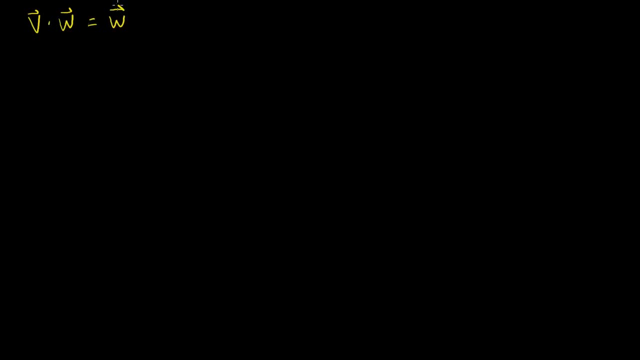 I want to prove to myself that that is equal to w dot v. And so how do we do that? Well, and this is the general pattern for a lot of these vector proofs- Let's just write out the vectors, So v will look like v1, v2.. 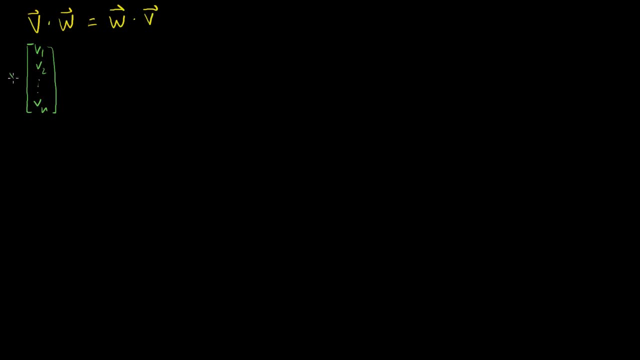 All the way down to vn. Let's say that this is equal to v And let's say that w is equal to w1, w2, all the way down to wn. So what does v dot w equal? v dot w is equal to- I'll switch colors here- v1 times. 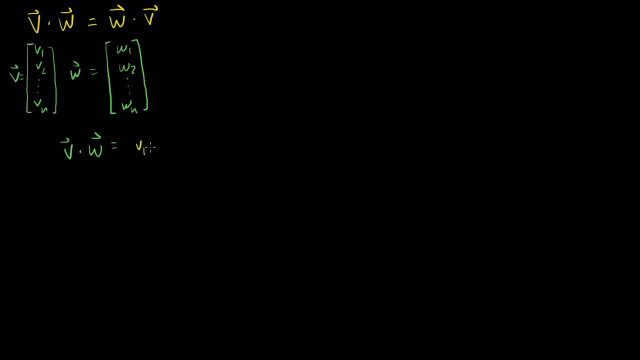 w1. Whoops, v1, w1. Plus v2, w2, plus, all the way to vn, wn. Fair enough, Now what does w dot v equal? Well, w dot v. when I made the definition, you just multiply. 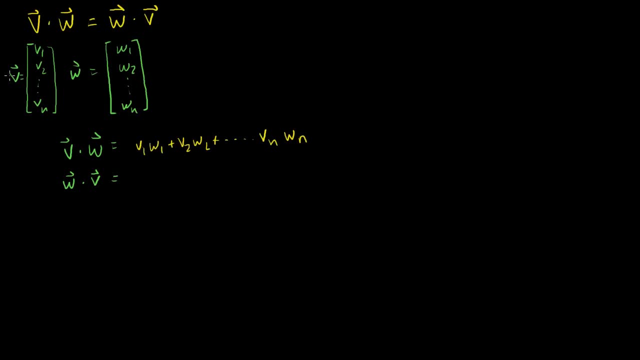 the products, but I'll just do it in the order that they gave it to us. So it equals w1, v1, plus w2, v2.. Plus all the way to wn, vn. Now these are clearly equal to each other because if you, 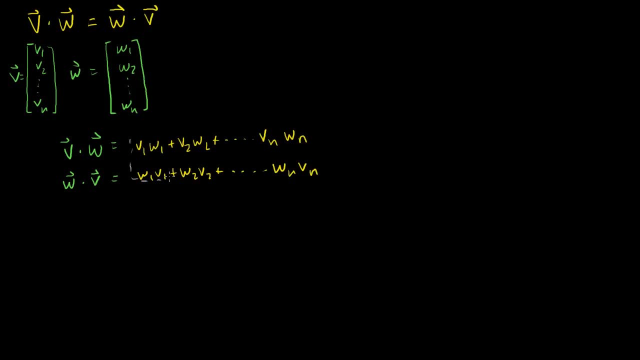 just match up the first term with the first term. those are clearly equal to each other. v1, w1 is equal to w1, v1.. And I can say this now, because now we're just dealing with regular numbers. Here we were dealing with vectors and we were taking 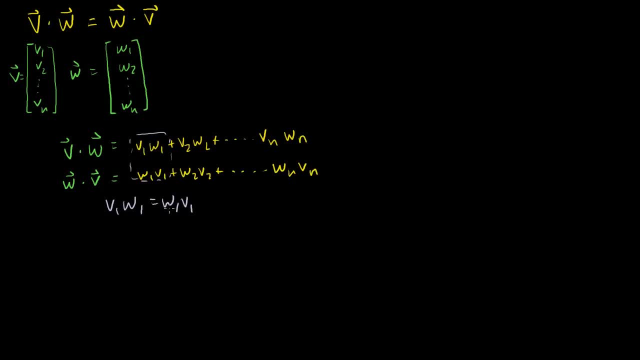 this weird type of multiplication called the dot product. but now I can definitely say that these are equal because this is just regular multiplication and this is just a community Commutative property of multiplication. We learned this in- I don't know when you learned this in. 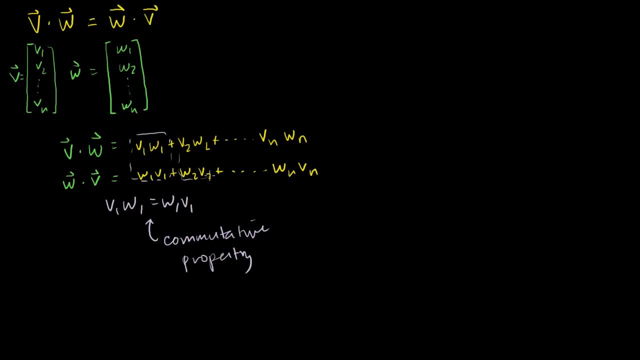 second or third grade. So you know that those are equal and by the same argument you know that these two are equal. Then you could just rewrite each of these terms just by switching that around. That's just from basic multiplication of scalar numbers, of just regular real numbers. 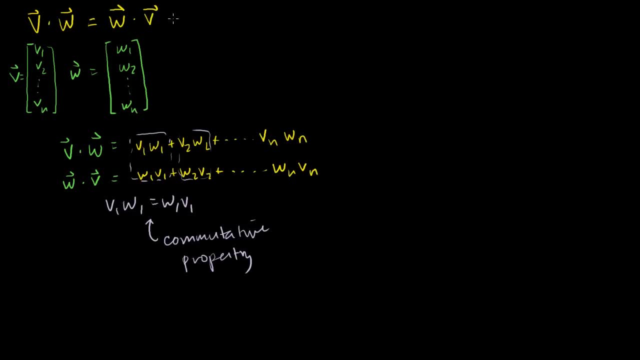 So that's what tells us that these two things are equal, or these two things are equal, So we've proven to ourselves that order doesn't matter when you take the dot product. Now the next thing we could take a look at is whether the 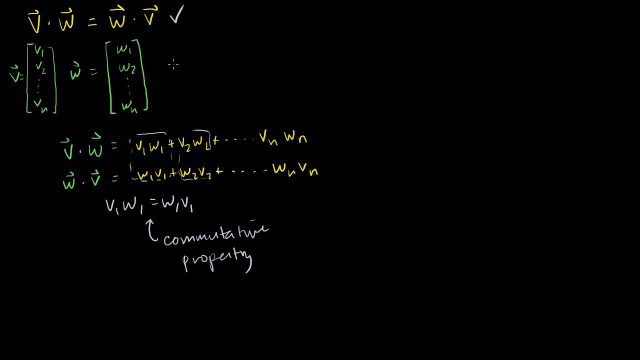 dot product exhibits the distributive property. So let me just define another vector x here. Another vector x, and you can imagine how I'm going to define it: x1,, x2, all the way down to xn. Now what I want to see if the dot product 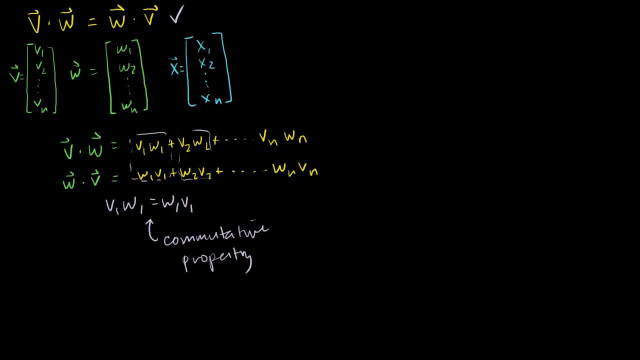 deals with the distributive property the way I would expect it to, then if I were to add v plus w and then multiply that by x, and first of all, it shouldn't matter what order I do that with. I just showed it here. 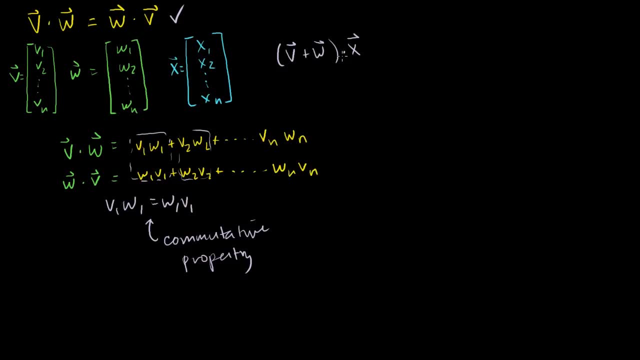 I could do x dot this thing. It shouldn't matter because I just showed you it's commutative. but if the distribution works, then this should be the same thing as v dot x plus w dot x. If these were just numbers and this was just regular. 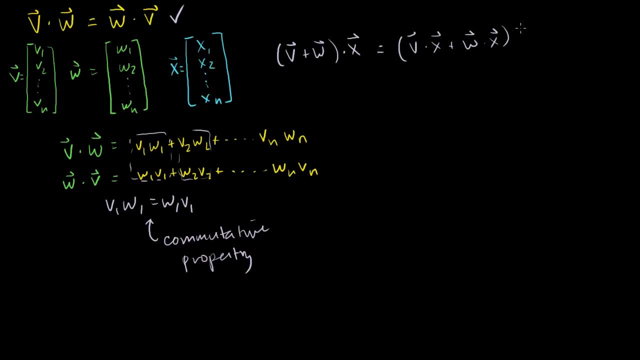 multiplication. you would multiply it by either of the terms, and that's what I'm showing here. So let's see if this is true for the dot product. So what is v plus w? v plus w is equal to. we just add up each of their. 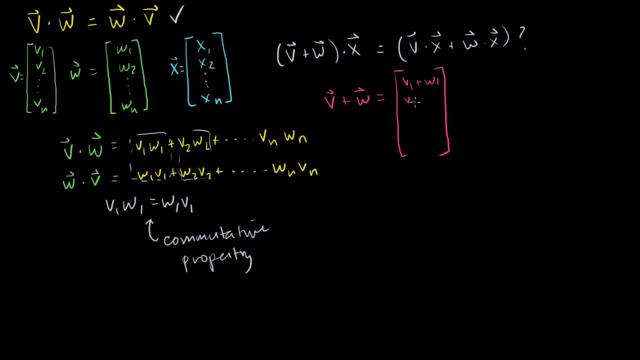 corresponding terms: v1 plus w1, v2 plus w2.. All the way down to vn plus wn. That's that right there. And then when we dot that with x1, x2,, all the way down to xn, what do we get? 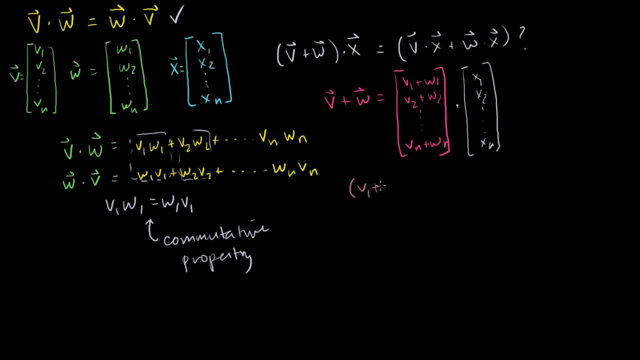 Well, we get v1 plus w1 times x1, plus v2 plus w2 times x2, plus all the way to x1. So we get vn plus wn times xn. I just took the dot product of these two. I just multiplied corresponding components and then added: 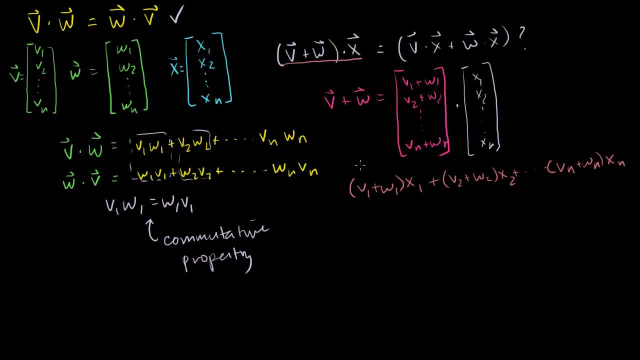 them all up. That was the dot product. This is v plus w dot x. Let me write that down. This is v plus w dot x. Now let's work on these things up here. What is v dot? Let me write it over here. 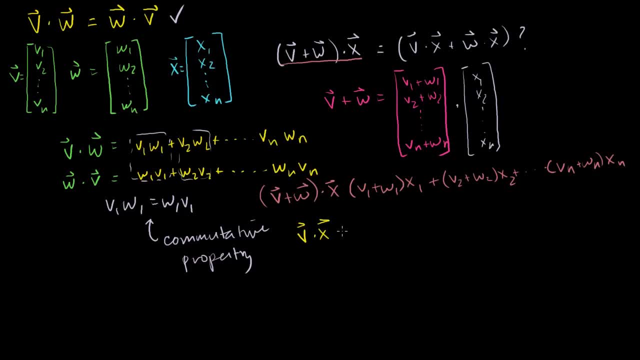 What is v dot x, v dot x, v dot x? we've seen this before. This is just v1, x1,, no vectors. now These are just their actual components, plus v2, x2, all the way to vn, xn. 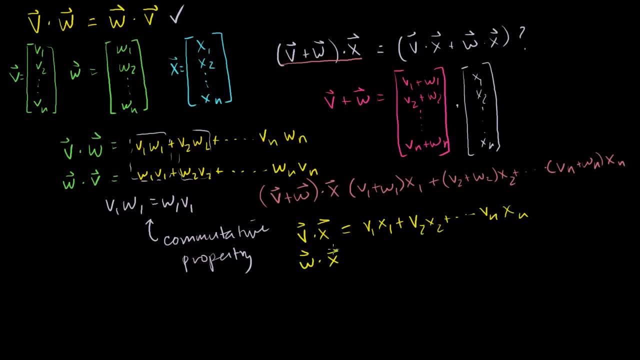 What is w dot x? w dot x is equal to w1, x1, plus w2, x2, all the way to wn, xn. Now what do you get when you add these two things And notice, here I'm adding two scalar quantities. 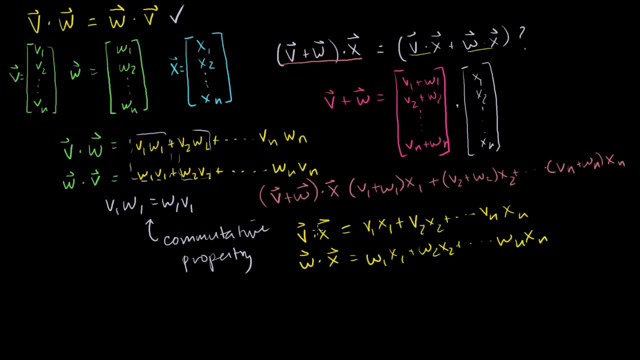 That's a scalar. that's a scalar. We're not doing vector addition anymore. So this is a scalar quantity. and this is a scalar quantity. So what do I get when I add them? So v dot x plus w dot x is equal to v1, x1, plus w1, x1,. 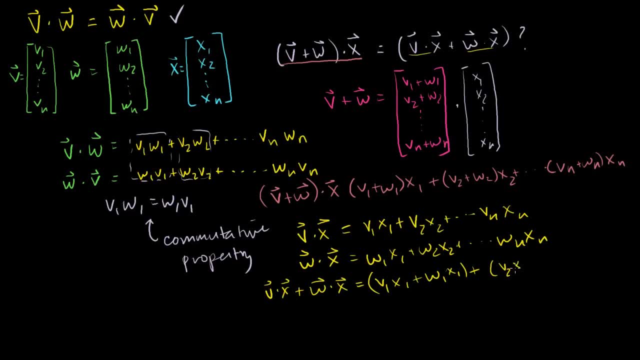 plus v2, x2, plus w2, x2, all the way. So that's equal to v2, x2, vn xn plus wn xn. I know it's very monotonous, but you can immediately see. 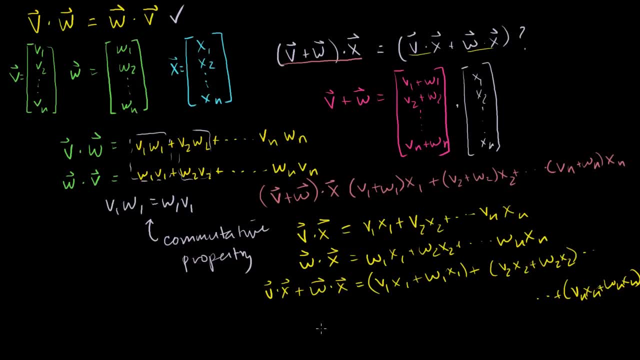 we're just dealing with regular numbers here, So we can take the x's out and what do you get? This is equal to. let me write it here: This is equal to: we could just take the x out. factor the x. 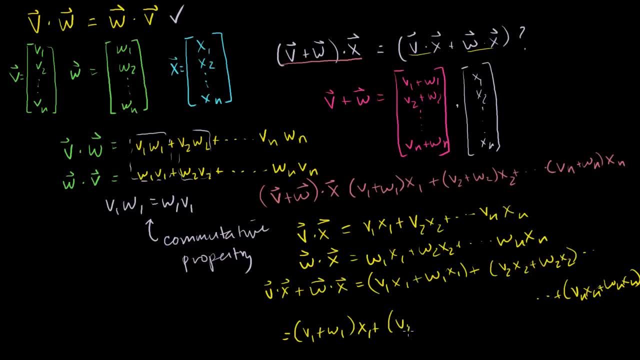 out v1 plus w1, x1 plus v2 plus w2, x2, all the way to vn plus wn, xn, Which we get, Which we see. this is the same thing as this thing right here. So we just showed that this expression right here is the. 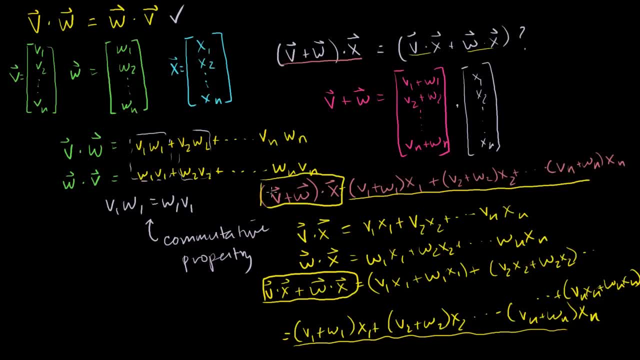 same thing as that expression or that distribution. the distributive property seems to or does apply the way we would expect to the dot product, And I know this is so mundane. why are we doing it? But I'm doing this to show you that we're building things up. 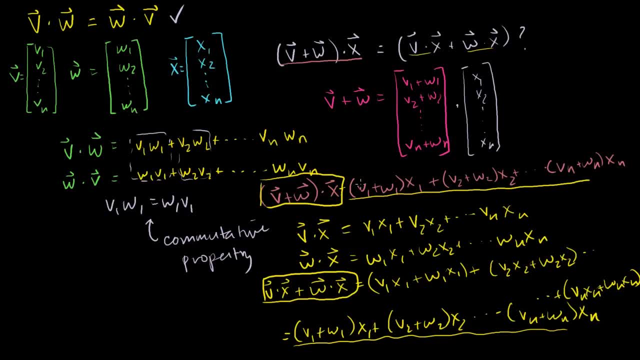 We couldn't just assume this. But the proof is pretty straightforward And in general I didn't do these proofs when I did it for vector addition and scalar multiplication- and I really should have- But you can prove the communitivity of it or for the 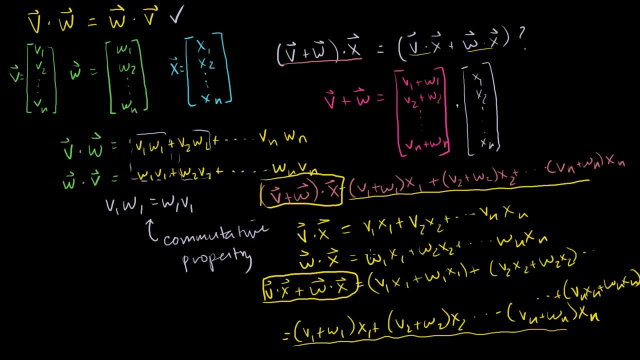 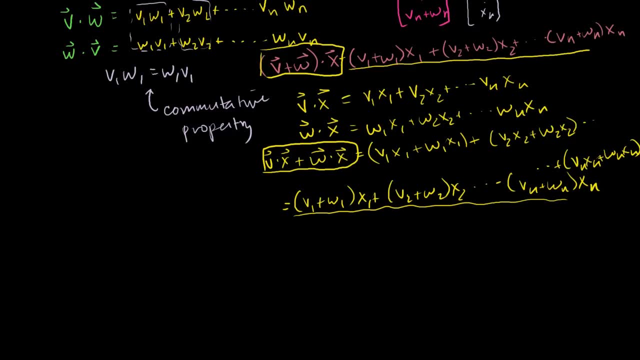 scalar multiplication, you could prove that distribution works for it, doing a proof exactly the same way as this. A lot of math books or linear algebra books just leave these as exercises to the student because it's mundane, so they didn't think it was worth their paper. 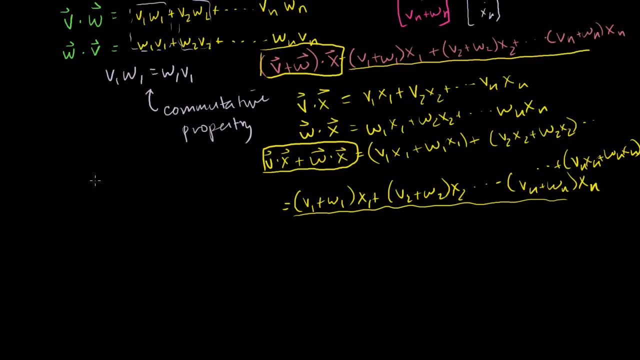 But let me just show you, I guess the last property, Let me just say associativity, the associative property, that doesn't matter where. So let me show you: If I take some scalar and I multiply it times v, some vector v, and then I take the dot product of that with w, if 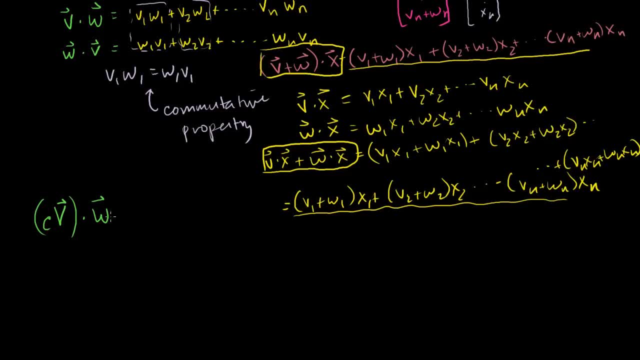 this is associative, the way multiplication in our everyday world normally works. this should be equal to- and it's still a question mark because I haven't proven it to you- it should be equal to c times v dot w. So let's figure it out. 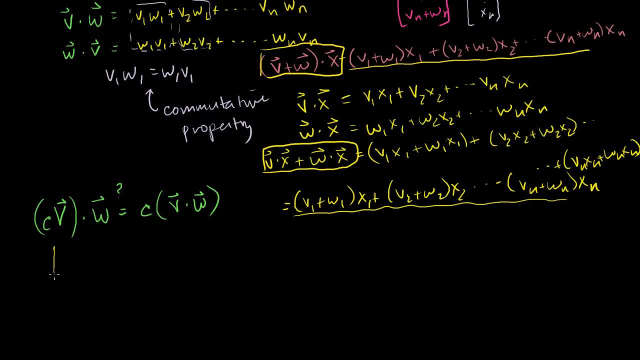 What's c times the vector v? It's c times v1, c times v2, all the way down to c times vn. And then the vector w. we already know what that is. so dot w is equal to what It's equal to this times the first term of w, so cv1w1,. 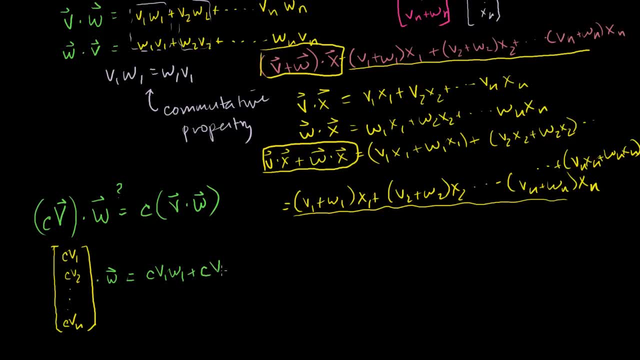 plus this times the second term of w, cv2w2, all the way to cvnwn. Fair enough, That's what this side is equal to. Now let's do this side. What is v dot w? I'll write it here. 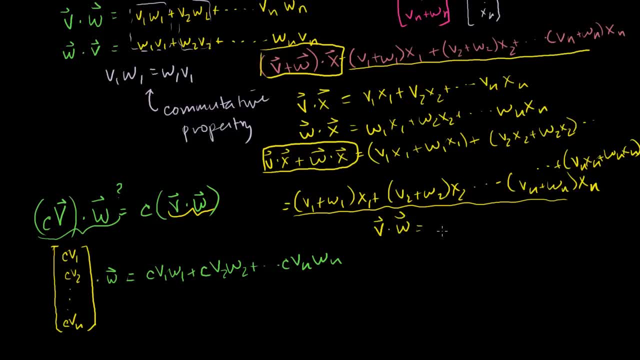 v, dot w. we've done this multiple times. This is just v1w1 plus v2w2, all the way to vnwn. I'm getting tired of doing this and you're probably tired of watching it, But it's good to go through the exercises. 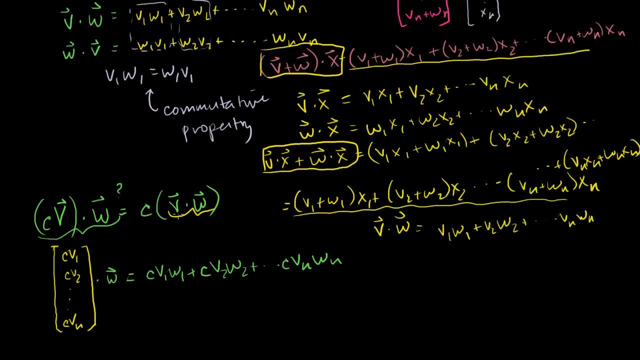 If someone asked you to do this now, you'll be able to do this. Now, what is c times this? So if I multiply some scalar Scalar times this, that's the same thing as multiplying some scalar times that. So now I'm just multiplying a scalar times, a big. this is.